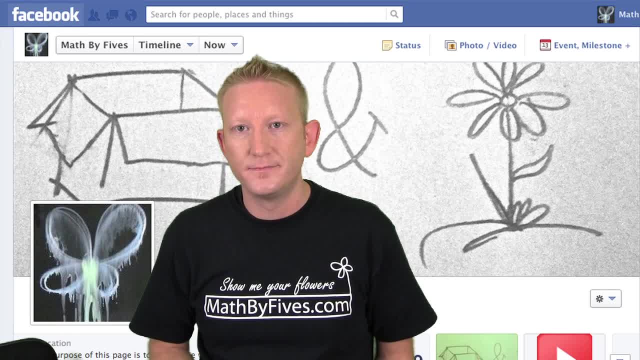 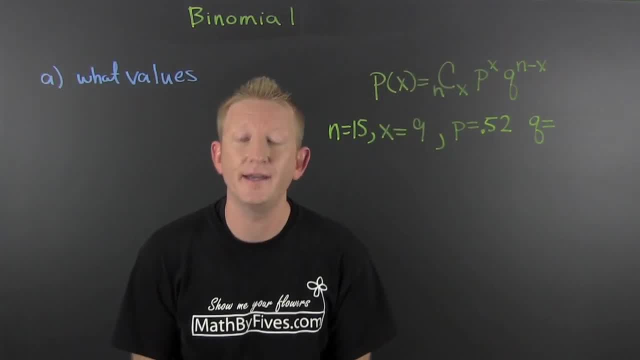 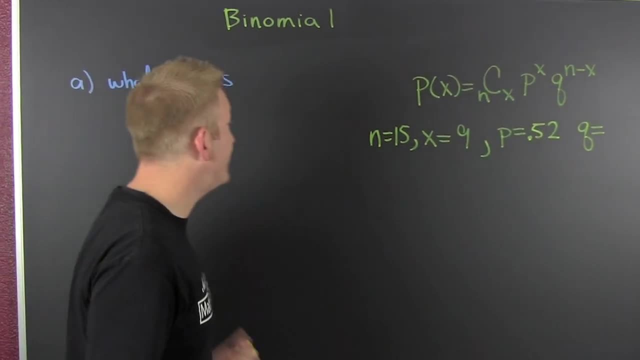 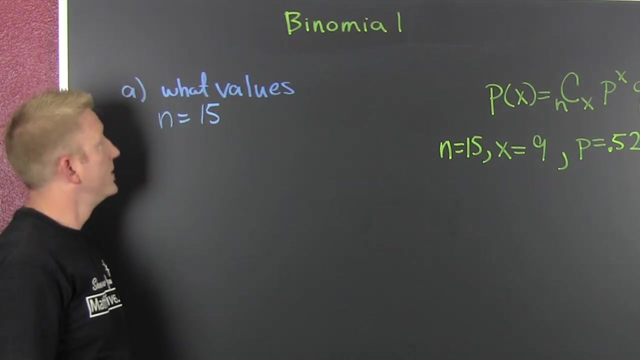 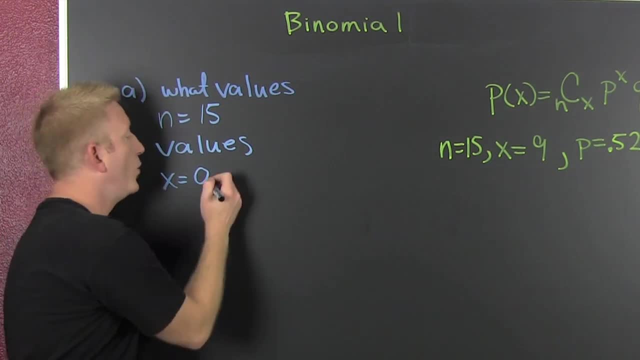 Zero, because none of them can have a Facebook account, or one of them can have a Facebook account, or two of them can have a Facebook account or- I've seen enough- 14 of them can have a Facebook account, or 15 of them can have a Facebook account. 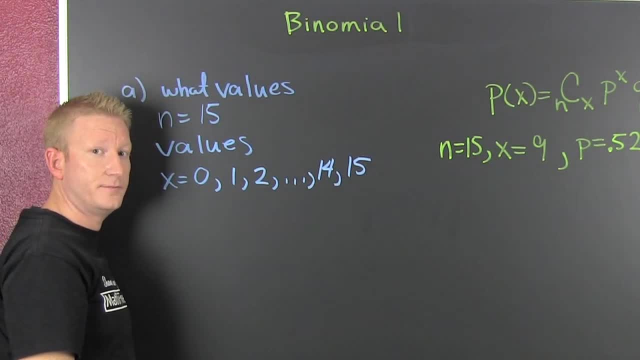 Out of 15, can 16 have a Facebook account? No, And that's why we stop right there, Liked it. If it was a Facebook page, you'd like it. It is. Let's go Over there, All right. next, 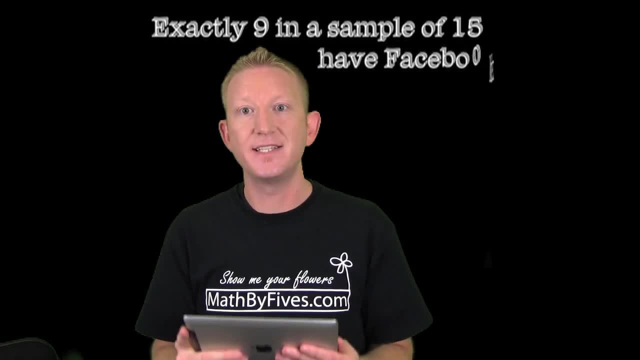 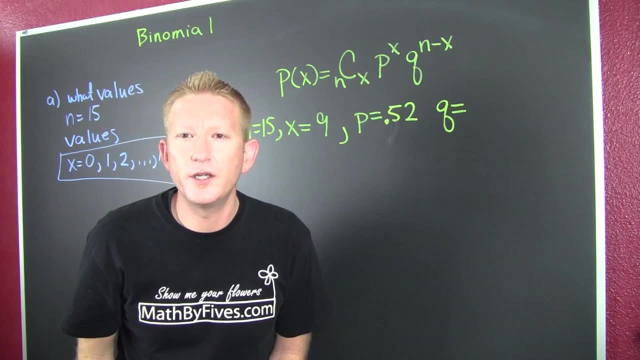 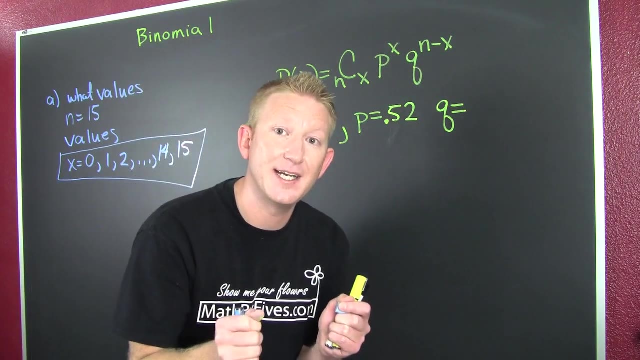 That exactly nine American college graduates- in a sample of 15, have Facebook accounts. Let's do that with the formula, Because now in Part B say they want to know the probability that you'll get exactly nine likes- well, not likes nine people with an account out of 15.. 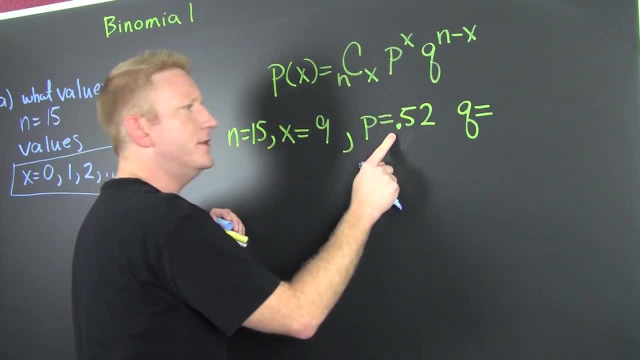 And they tell you the probability that somebody has an account is 15. 52%. How are we going to get Q? Well, P plus Q is equal to 1.. So you can take 1 and subtract that off. Or you can ask yourself, oh self, what do I add to 52 to get 1?? 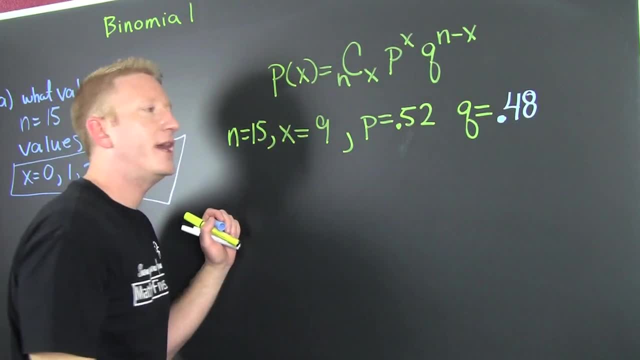 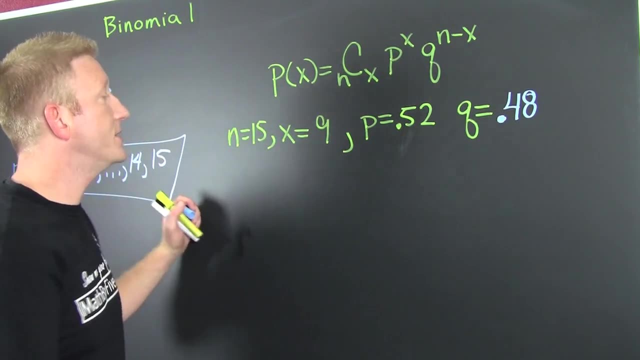 And that's 0.48.. Great, And now we're going to go and plug it in. plug it in: It's going to make the binomial distribution smell fresh. So this is the probability of exactly nine people having an account. 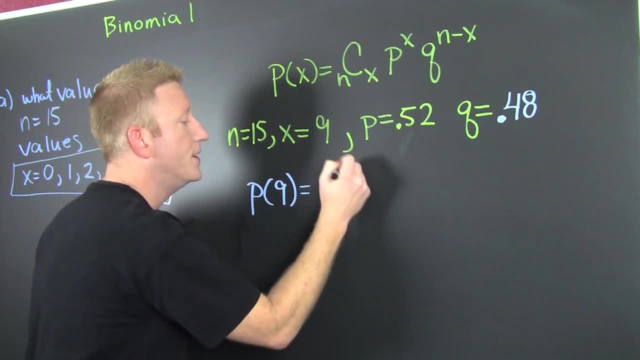 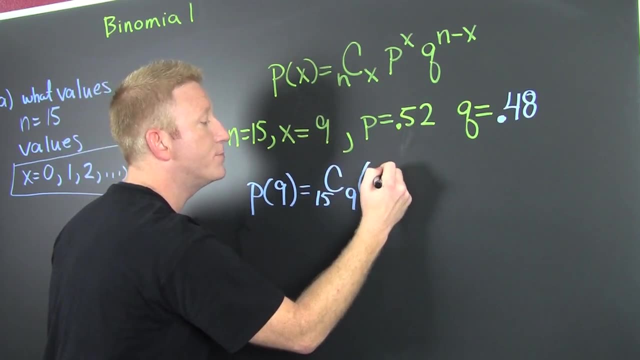 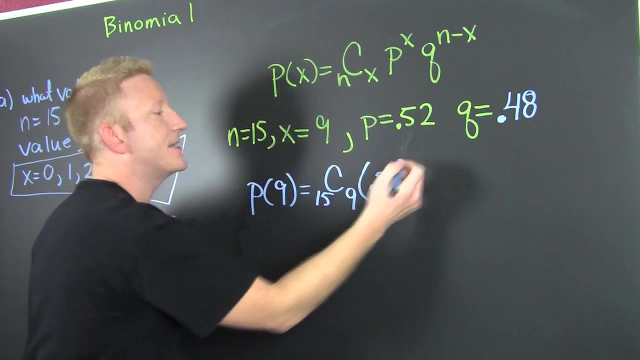 So let's account for the total number of people. That's the combination of 15 things. Choose nine, And then this is 0.52.. How many successful? How many successes are you looking for? You're looking for nine successes.